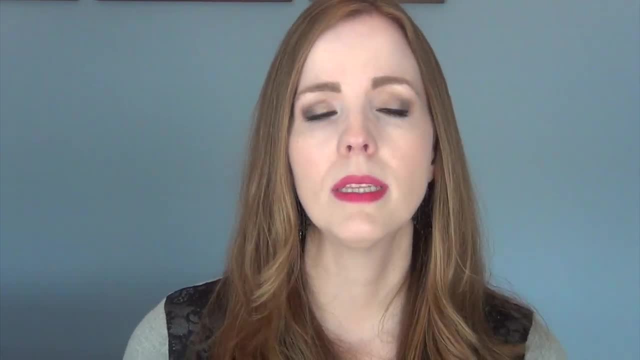 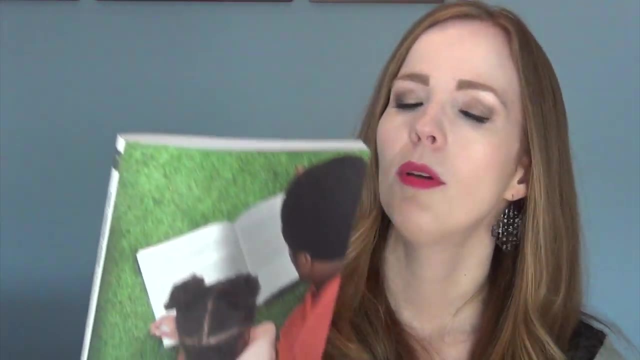 program. So I showed these books in that video, but I really wanted to do a little bit more of an in-depth video about the first language lessons book in particular. We've been using it now since the middle of August, so it's been a few months now, and I really have enjoyed. 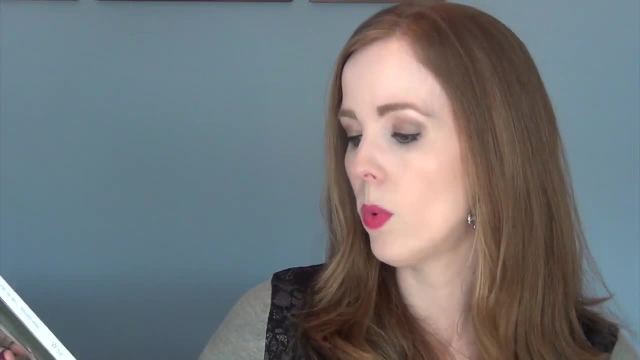 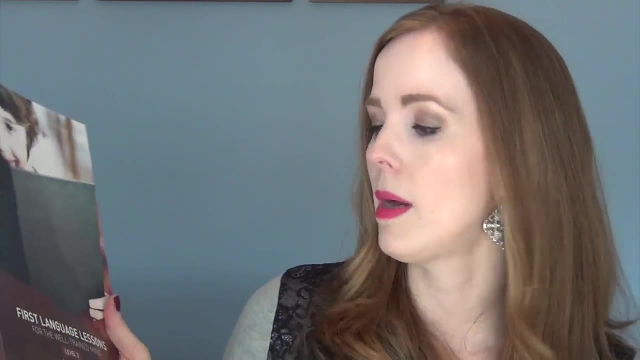 this book. This is the First Language Lessons for the Well-Trained Mind, Level 1.. And then I actually loved the first one so much- and we're going through it so quickly- that I actually just recently purchased the First Language Lessons for the Well-Trained Mind. 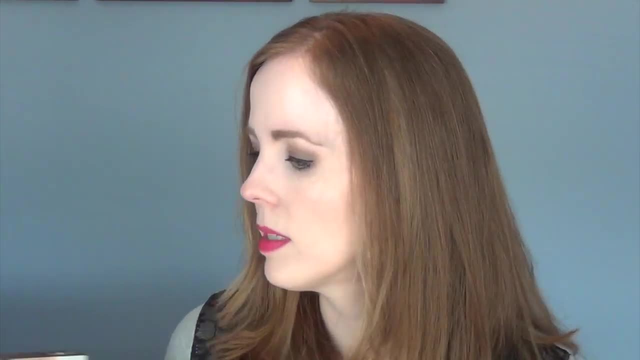 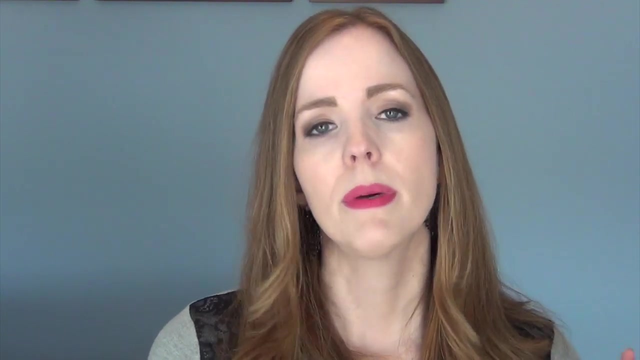 Level 2.. So we're not quite ready for that one yet, but I wanted to kind of explain a little bit more about this book and the books that we're using with it. I don't have those other workbooks to show you up here, but I will link my first graders curriculum video. 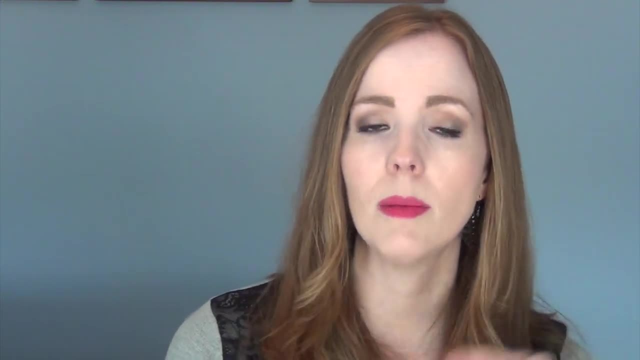 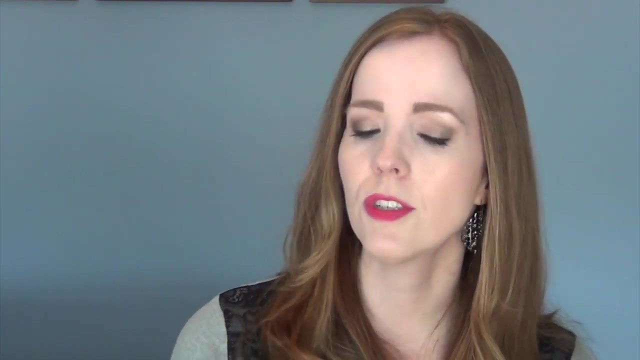 down below. You can watch it and see the workbooks And I will also link the books in the description box below And I have something to say about that. I do have something to say about those workbooks in a minute, but first I want to 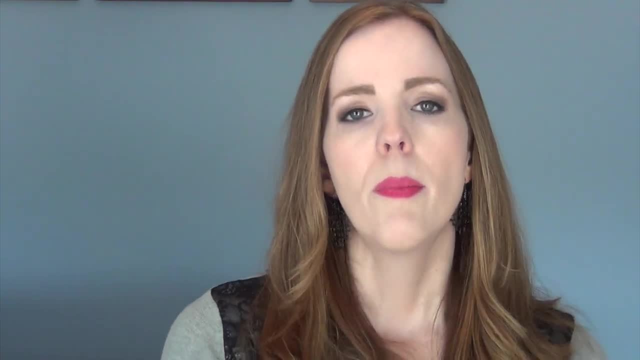 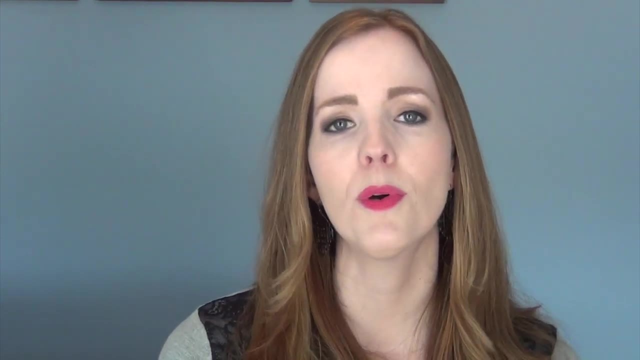 talk more about this. I really wanted to find a program for my first grader that really basically told me what to teach her and when to teach it. I've mentioned before I need a little bit of a hand-holding when it comes to homeschooling. I do have a book that I 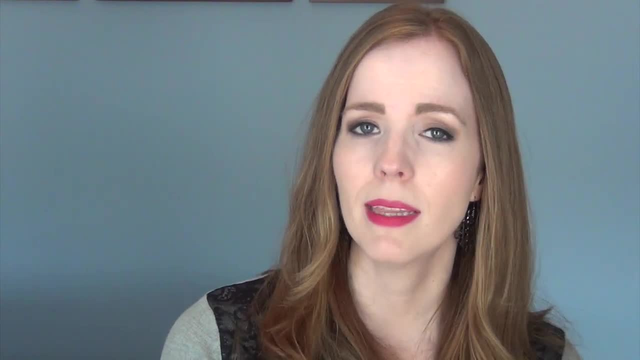 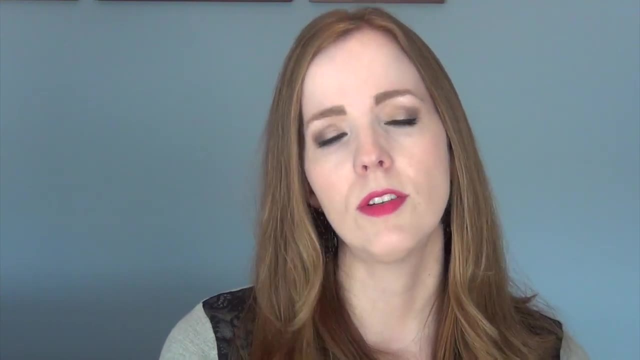 use as far as a grade-level framework or guideline of what each child in a certain grade should kind of be learning. I don't want to say should be learning, but basically what, like if she was in public school first grade, basically what she should know for that level. I don't 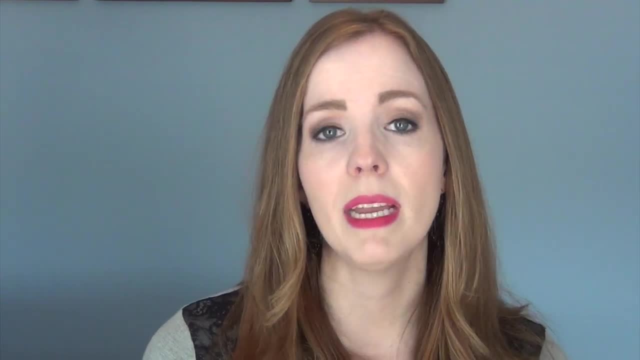 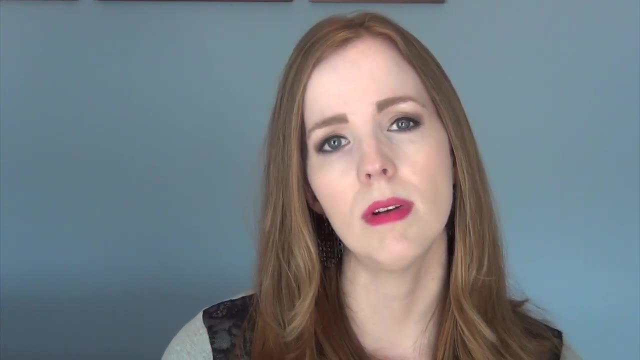 follow it to a tee, because we do homeschool and I do like to pick and choose what I think she should learn when. But for the most part I do like to try to follow that too loosely follow that, And so a lot of what I was finding are the basics of grammar. So you've got nouns. 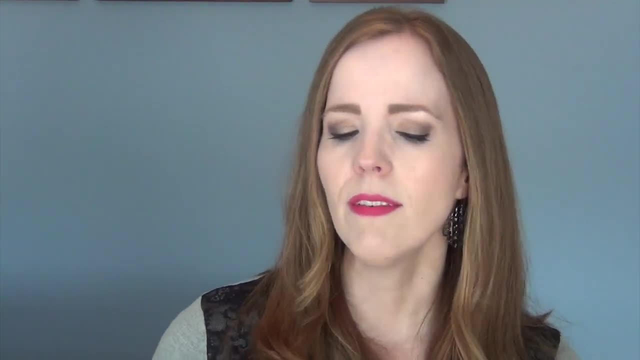 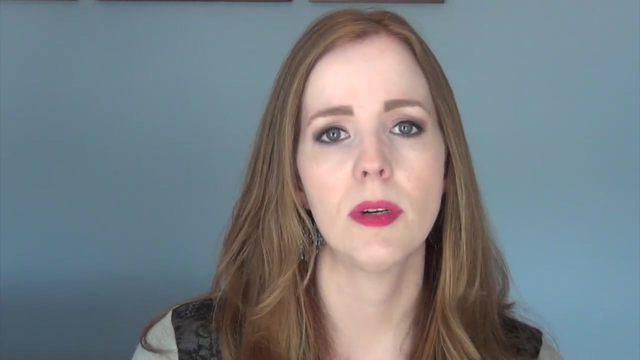 and pronouns and adjectives and proper nouns and all those things And I forgot where I had heard about this book. but I gave it a shot and I really have loved it. The only thing I will say that could be a downside for this book is the lessons. 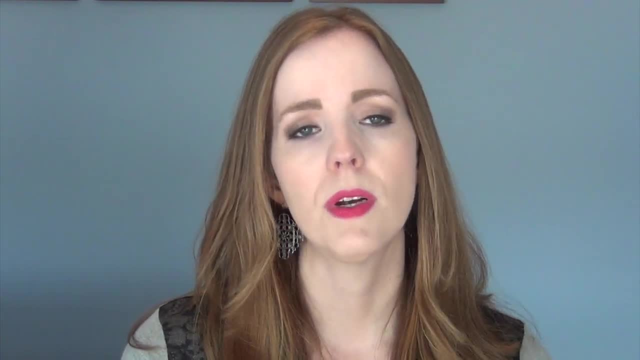 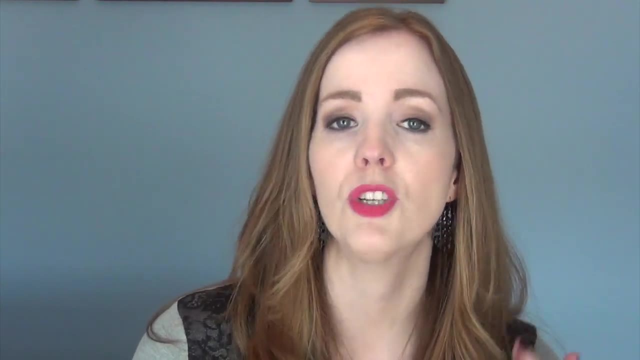 are very repetitive And it's very scripted as far as, like you as a teacher, say this and you expect your student to say this, And if they don't say it that way, you kind of correct them gently, you know, with the way they're supposed to respond, And so this whole teaching. 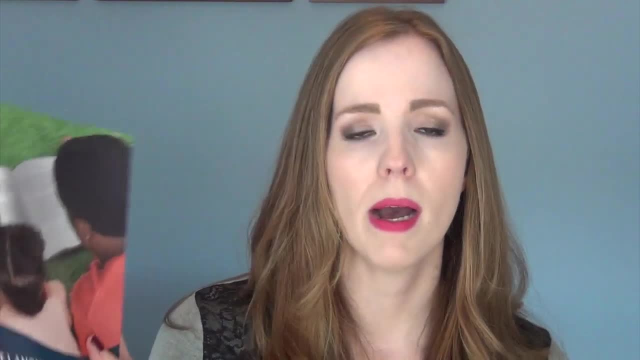 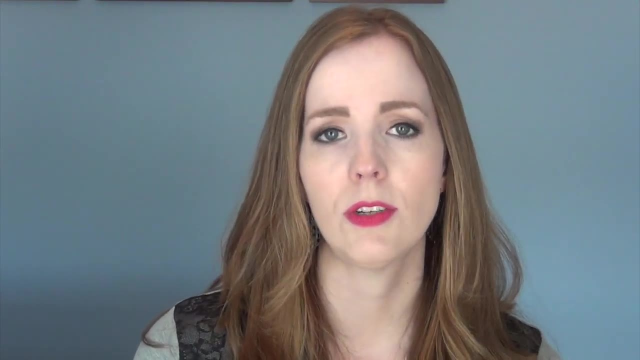 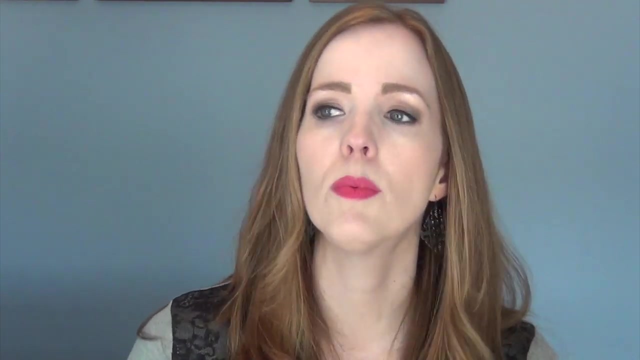 and this whole technique is basically based on- and it's the well-trained mind theory of teaching. So it's a lot of memory work and a lot of repetitive exercises, So but I think there is value in that and I do think it's important and I have found that it's necessary to keep. 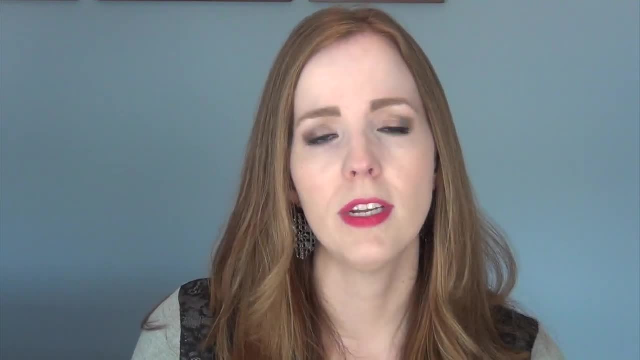 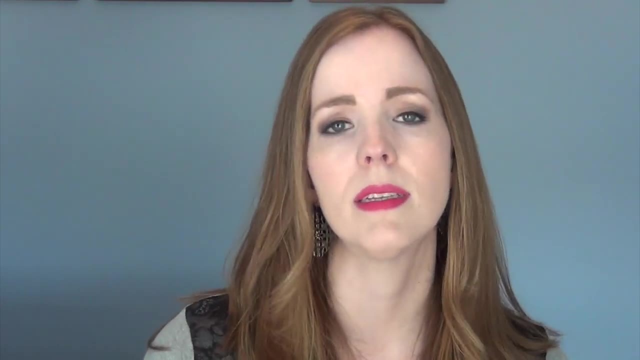 reviewing these terms, these new things to her. You know they're in first grade. I just recently learned their letter sounds and their vowel sounds and how to write and now you're throwing things at them like nouns and pronouns and verbs and things like that. So a lot of. 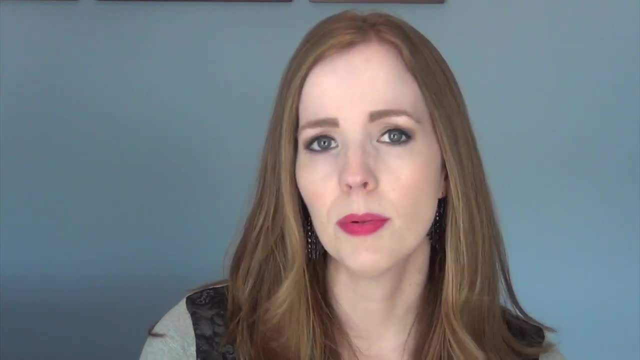 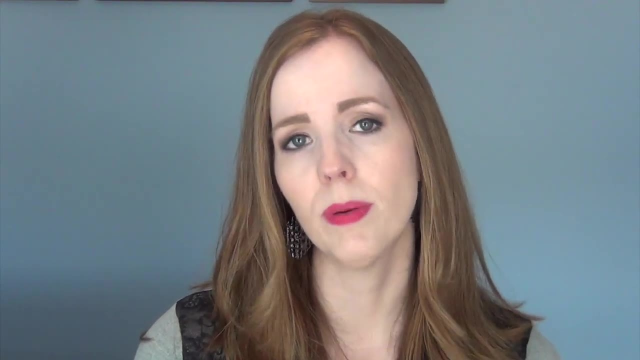 repetition sometimes is necessary. whether it's always the most fun approach or not, I don't know, But it seems to work. It's been really effective for her and I really have liked having a scripted style teacher's book, because that way I know. if I don't know what to say, I have it down. 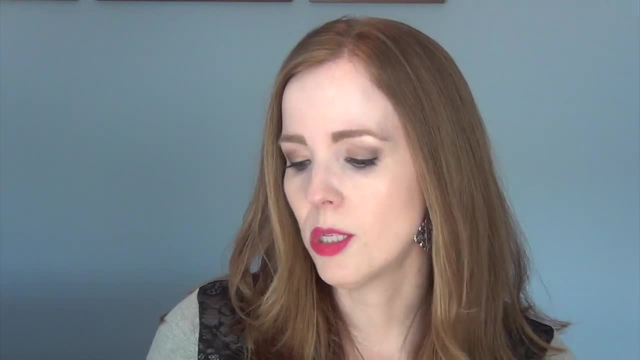 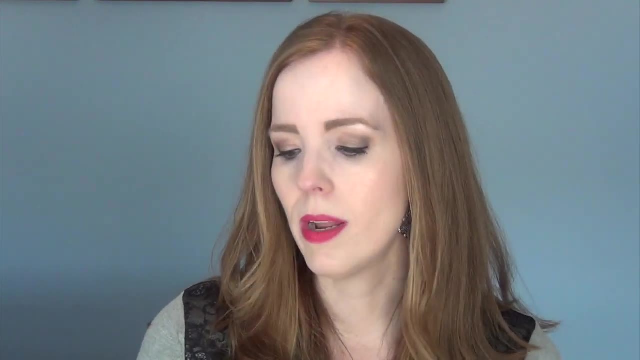 here that it's going to tell me what to say Now. the only thing that we don't do in this book is they have poetry memory work in every lesson, And I understand the value of that, but I just don't think right now it's necessary. 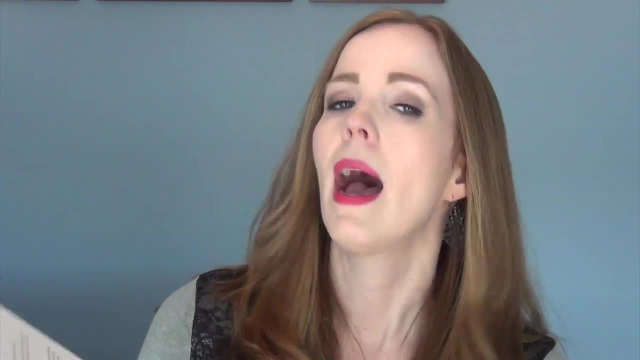 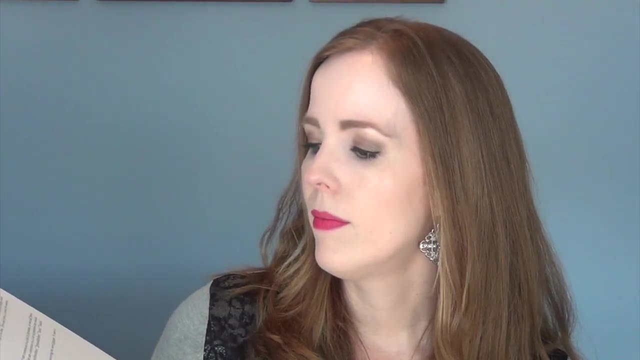 for us. So we are not doing the poetry memory work. I'm basically using this book as a guideline of what to teach her in grade one and also how to teach it. It's got your spot as an instructor and what the student should say, And it just goes on that way. You know we. 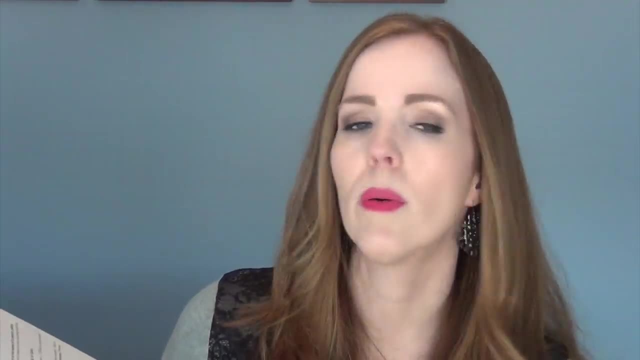 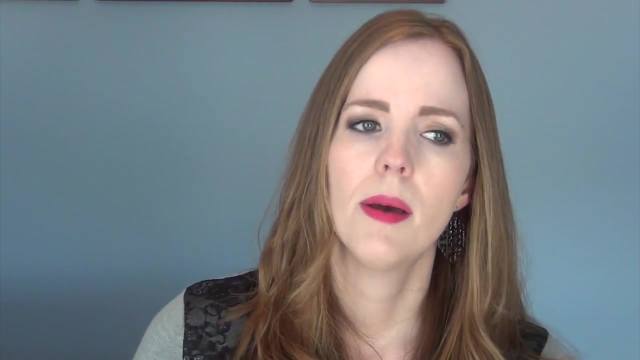 skip the. here's a poem, we skip that. And if it mentions you know, review the poem, we just skip that part. It doesn't bother me that I'm not using this book to its full potential because we're not working on the memory work. It doesn't bother me. This is 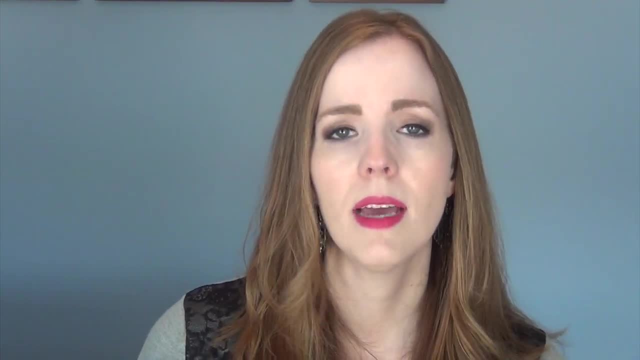 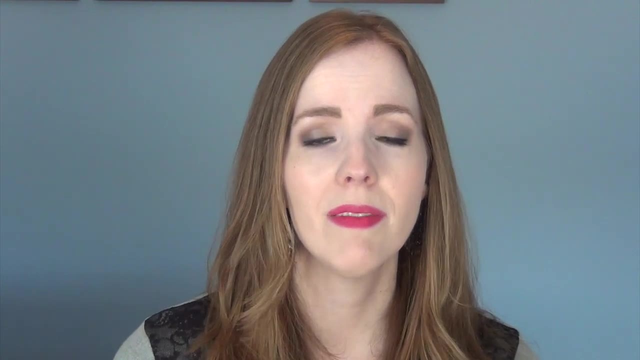 a really inexpensive book and I really like having it as a path and a guide to follow. The lessons are very repetitive and they do take a lot of time. I'm not going to spend much time on that, But the reason that it's so nice to have that repetition- because in 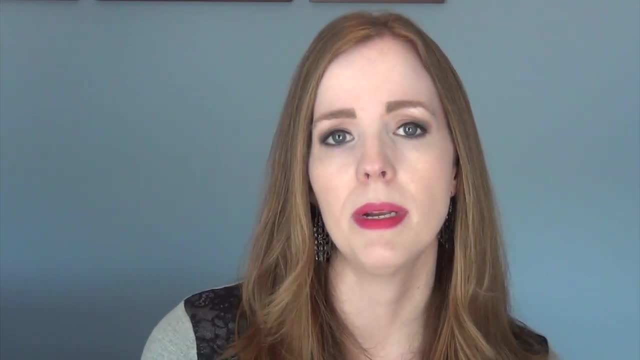 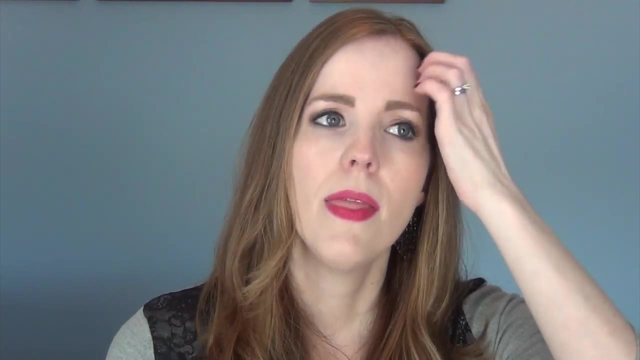 the meantime, they're using different examples of common nouns and different examples of proper nouns in each lesson. So, like you learn about common nouns, you talk about that for a long time and then, when you get to proper nouns, it talks about their name and their. 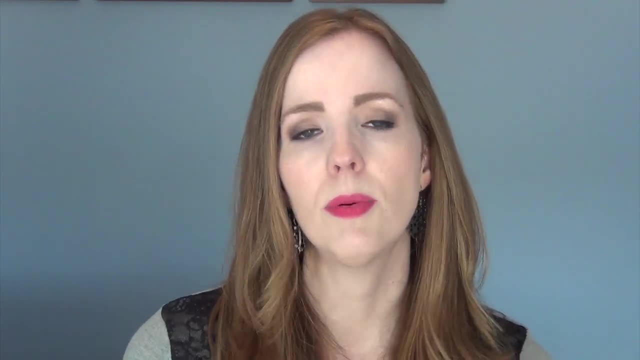 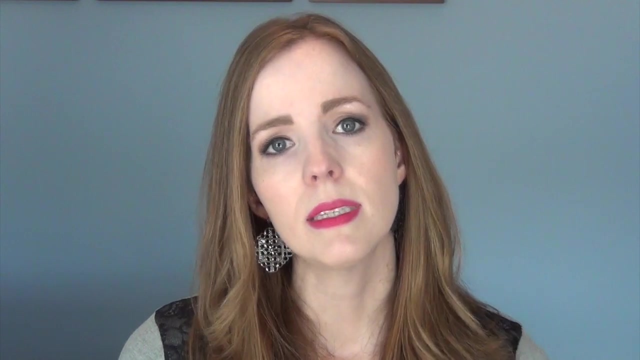 first and last name. So then they work on days of the week. It brings in days of the week talks about how the days of the week are proper nouns, and so then they learn their days of the week in order. they talk about months and seasons, how that. 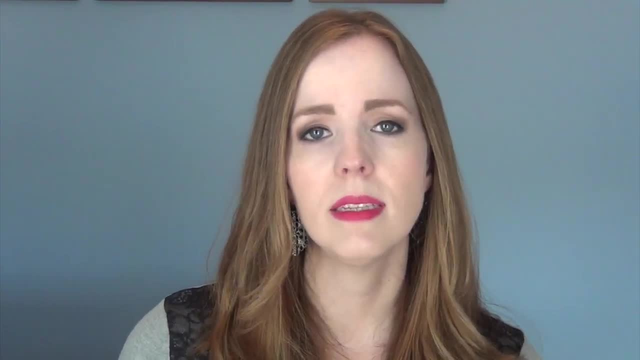 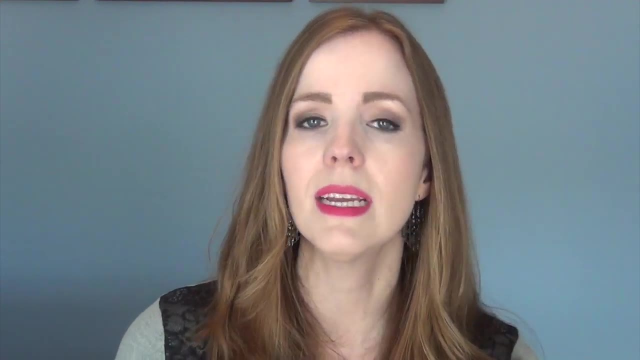 they are proper nouns and you learn those in order. when it combines what you're already talking about and reviewing like pronouns, but it also combines it with learning initials or the days of the week or the month of the year, things like that. I really love how it combines those and it's been a really 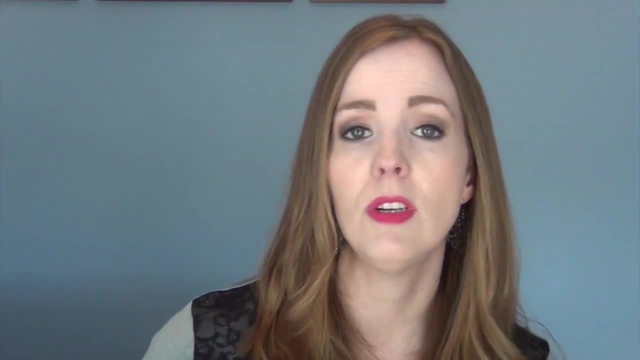 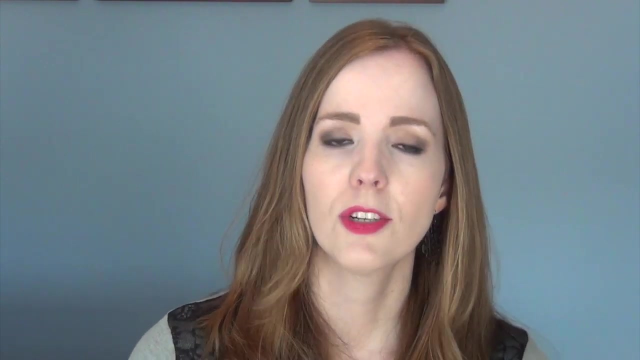 great book for us so far. we're already over halfway through and we just started this in the middle of August, but now we have been using some workbooks in combination with this. that's extra practice for her about like pronouns and verbs and capitalizing the first letter of a sentence and capitalizing the first. 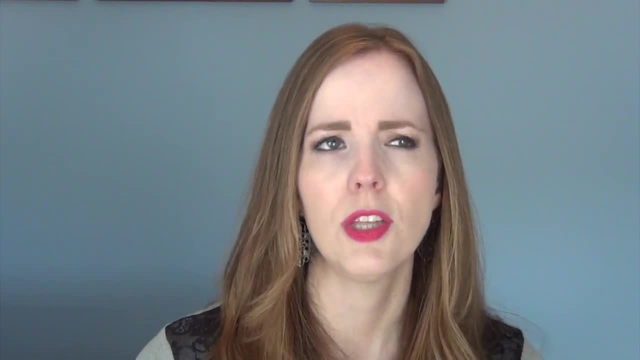 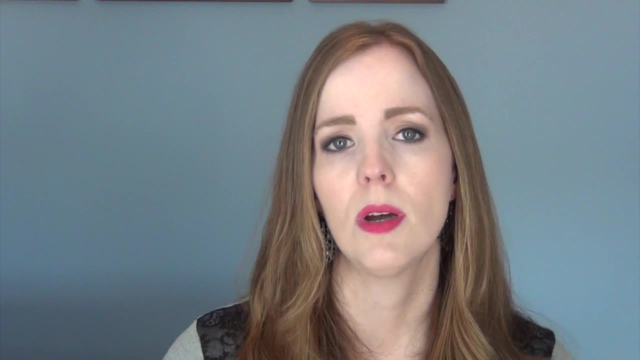 letter of a proper noun. we do have two workbooks that we're using- actually three workbooks that we're using for that- but I'm still finding that it's not enough practice. now I'll link the three workbooks that we have down below. you could definitely get those and use those in combination with this book, and they're 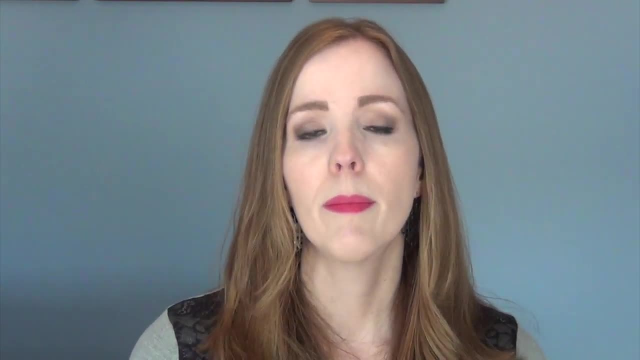 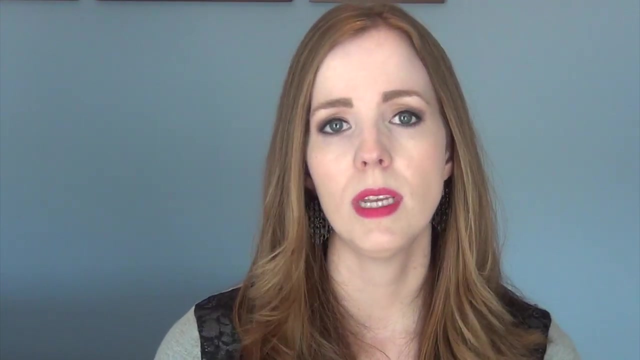 a great, a great marriage of you memory work and review, but then also having worksheets to do. I just think we need a lot more practice. I'm trying to find something else that we're going to be using in combination with this book, because I definitely want to give this. 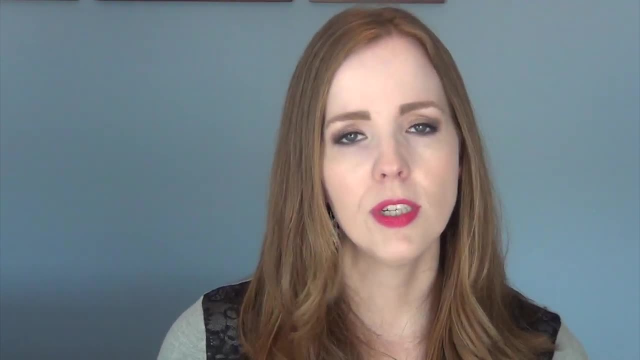 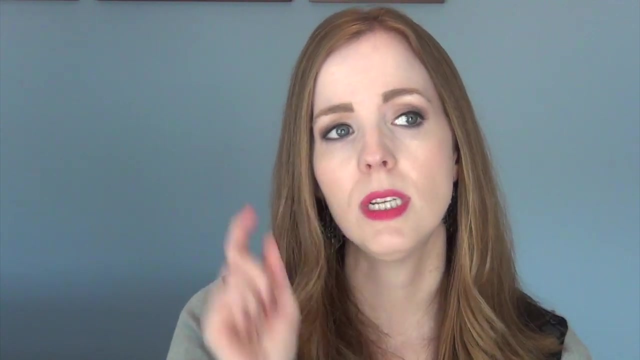 up. so I'm looking into the Moffat girls. I mentioned her teachers pay teachers store before. she's got great math and reading and all different types of activities. you can purchase things. she does have a language arts bundle for second graders which is all about adjectives and adverbs and nouns and all. 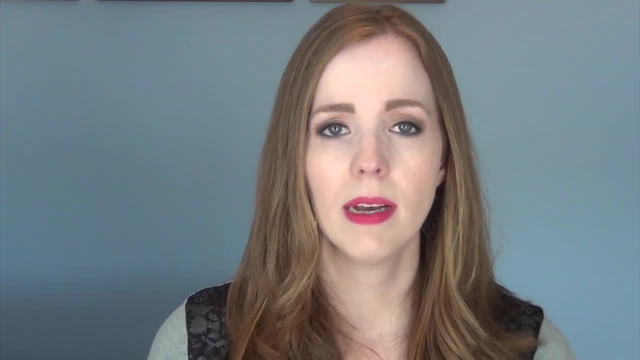 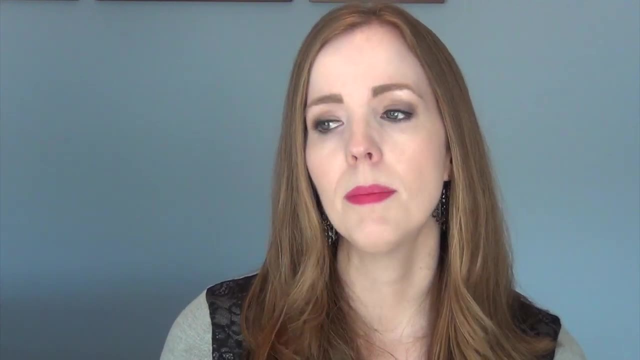 that stuff. but that is for a second grader. it's on a second grade reading level and since my youngest is in first grade she's not quite ready for a lot of the worksheets in that package. but I do know that Annie from the Moffat girls is. 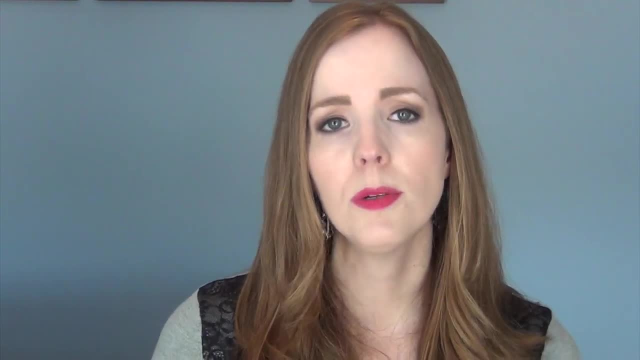 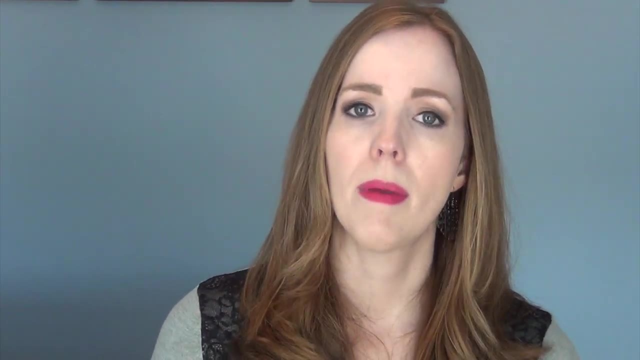 making a language arts bundle for first grade. it's supposed to be out at the end of November, so planning, I'm getting that and using it and I will be doing a review video about that in the coming months, but for now, I just really wanted to share this book with you and I highly encourage you if you don't have a. 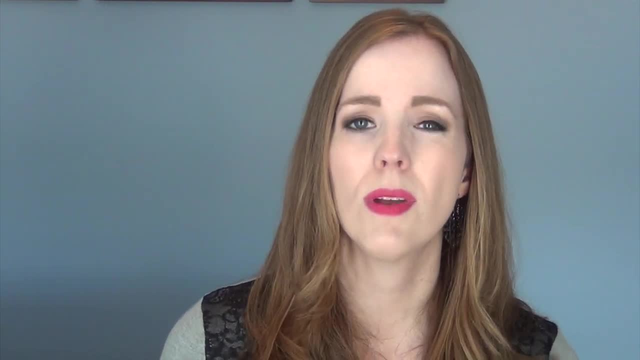 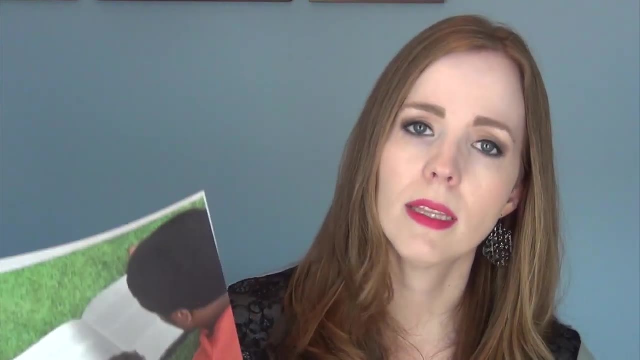 language arts program or you're just starting out, you really don't know where to start and you kind of like this sort of scripted repetitive memory work type approach. I think you'd really like this book. I will have links for all the books I talked about in the description box below and make sure you stay tuned.